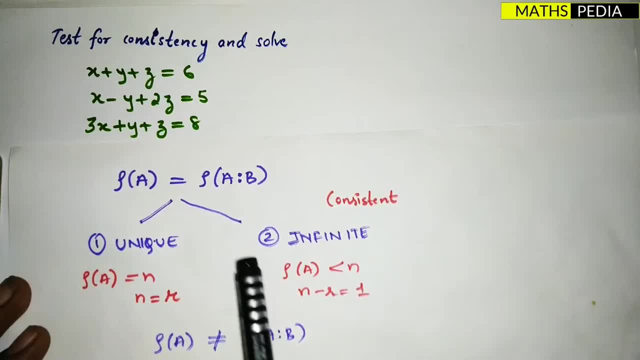 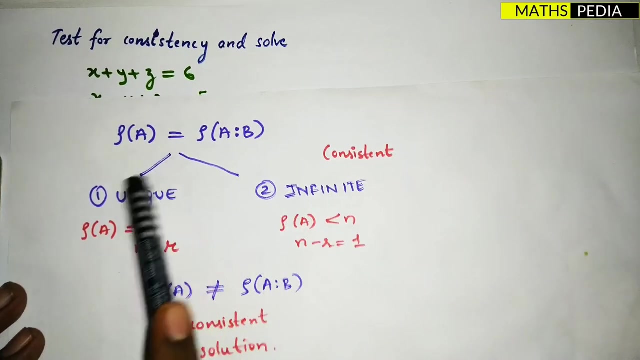 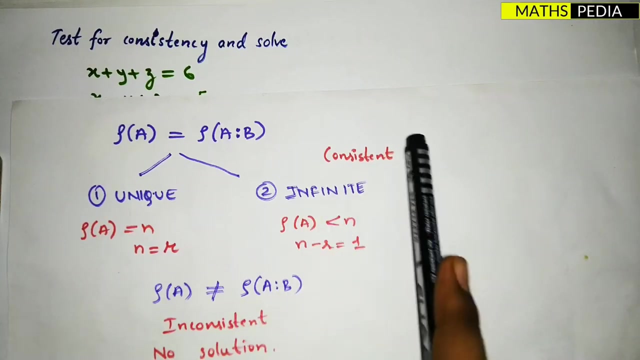 rank means you have to reduce the matrix into what echelon form and you have to see- and matrix a will be the this part, okay, I'll show you that thing- coefficient of XYZ and augmented matrix rank. also, you have to see if it, if both are equal, that means matrix a rank and augmented matrix rank are same. then we can say there are two possibilities. one is they can have unique solution. another one is infinite solution. and one more thing: that is consistent, okay, consistent, and we have to see whether it is unique or infinite. 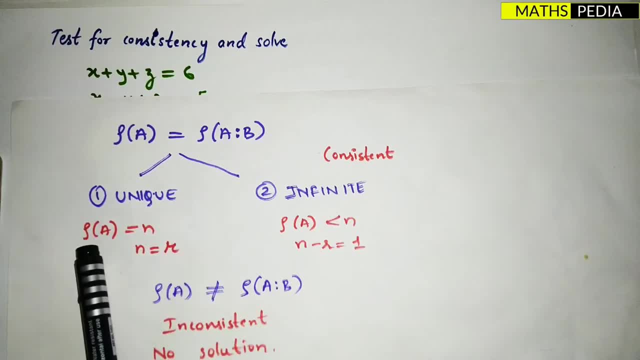 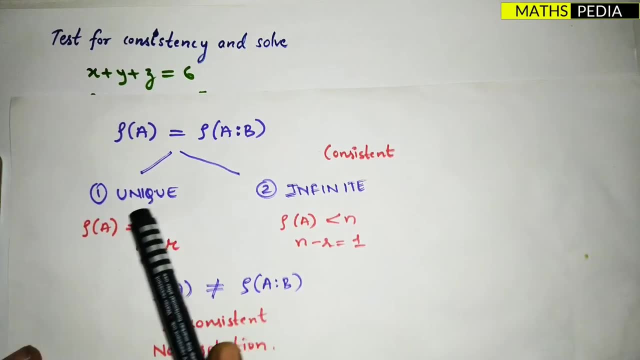 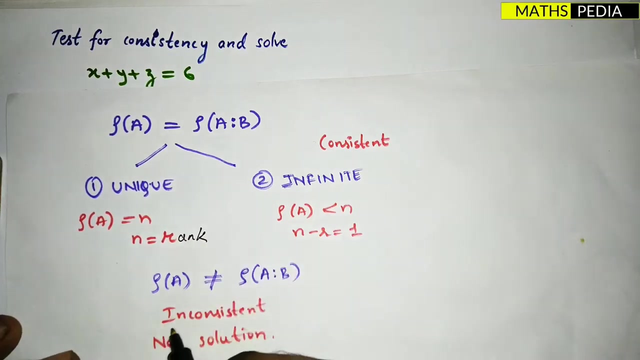 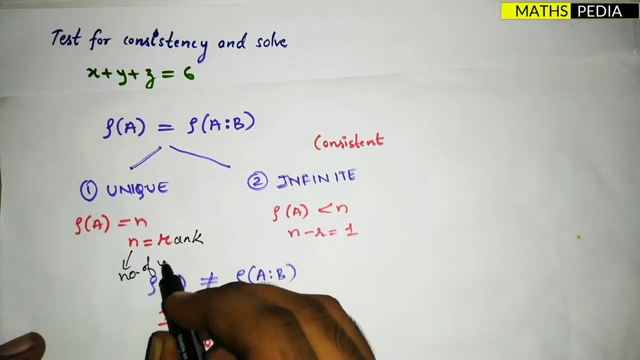 unique means the rank of a, which is equal to rank of this thing, will be equal to n. n means number of unknowns. remember, n is number of unknowns, n equal to r. r basically means rank, this is rank and this is number of unknowns. or we can say number of the variables, we can say unknown variables. okay, number of unknowns, and here infinite. 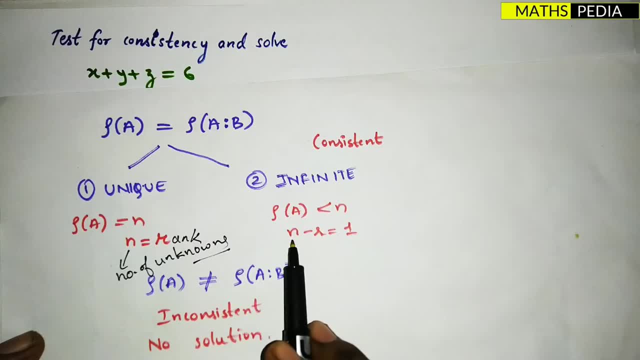 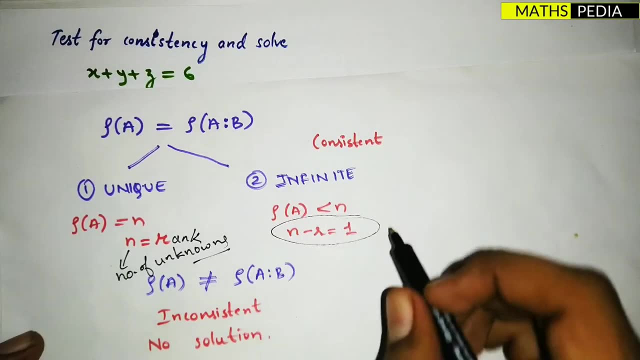 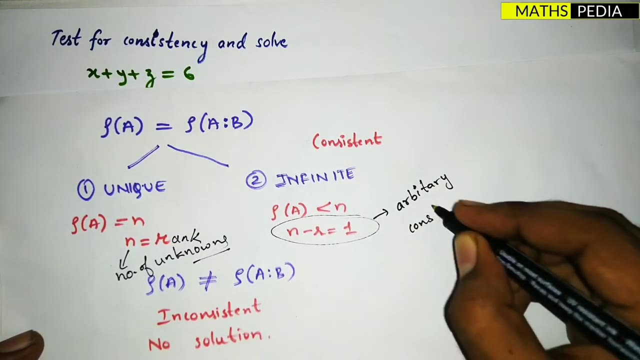 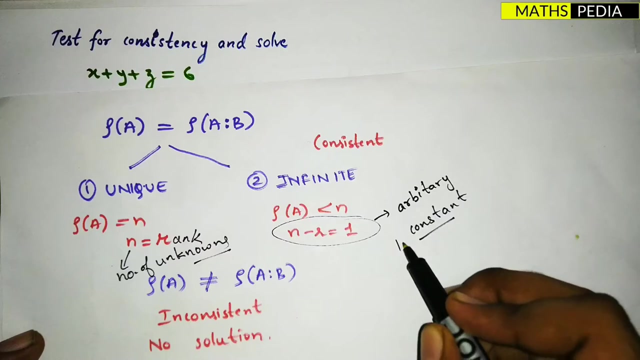 rank means rank of a should be less than- and that is n minus r- should be equal to what one now here n minus one are. that's meaning of this is nothing. but here we are going to check whether we have to assume anything as arbitrary constant. okay, arbitrary constant, we have to assume, or not, any of the variables, whether we have to represent it. is it as arbitrary constant or not? for that n minus r you have to do here also you can. 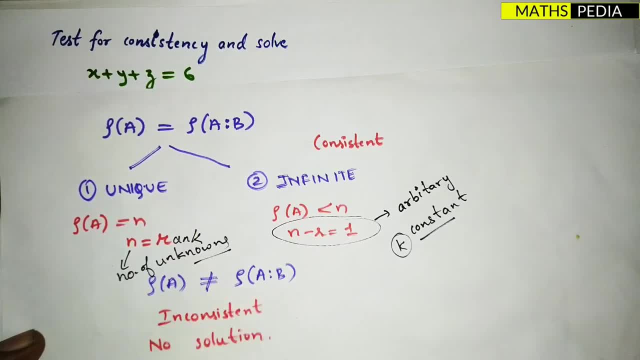 do n minus r, since both are equal, it is equal to zero. okay, here, in this case, rank of a, which is less than n. therefore n minus r will be, we have to see. okay, that depends, this value depends, this value depends. okay, arbitrary constant. but if it is n equal to minus 3 and a rank is 2, then it. 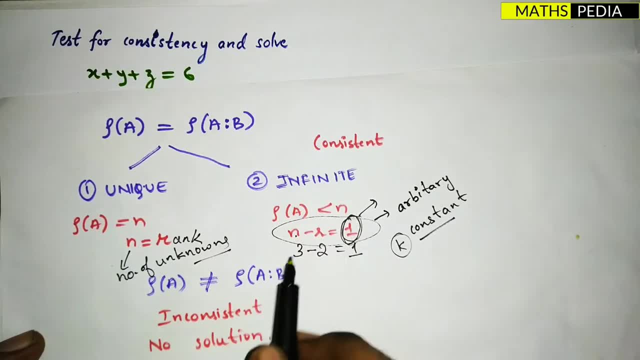 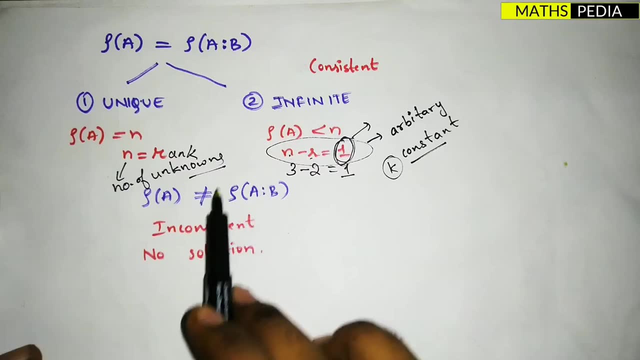 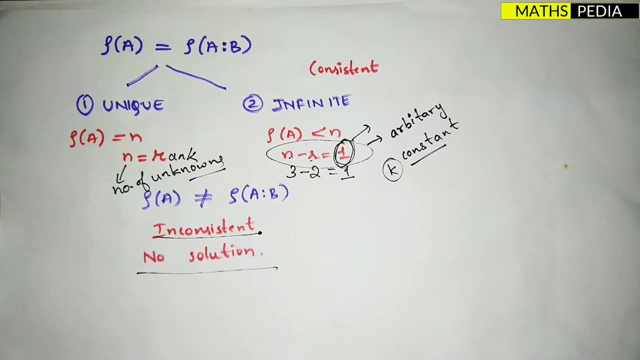 is equal to 1.. if it is some other values, it depends on the n and r values. okay, that we'll see now. the last one is the rank of a should. if it is not equal to rank of augmented matrix, then it is inconsistent and it has no solution. simple, see these things with. 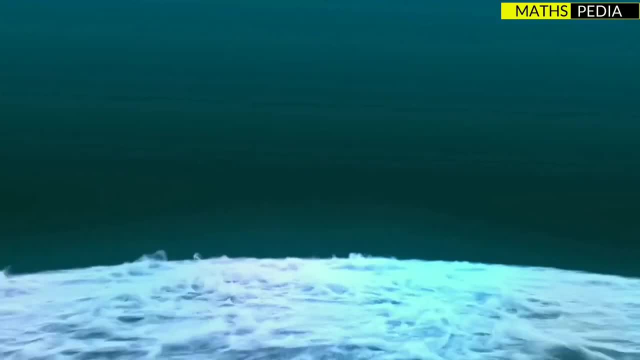 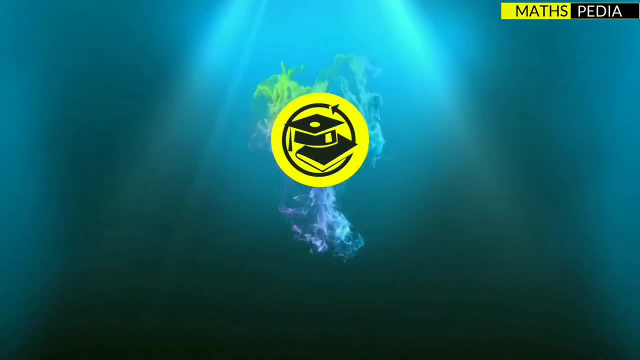 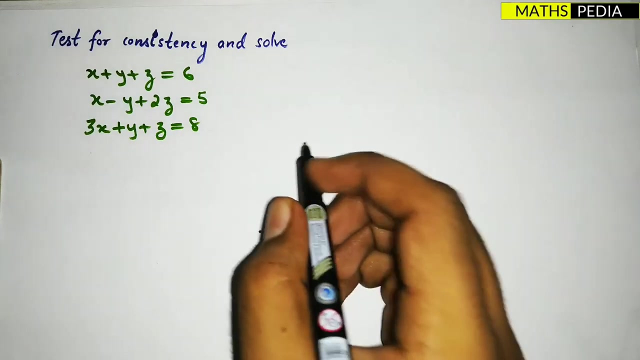 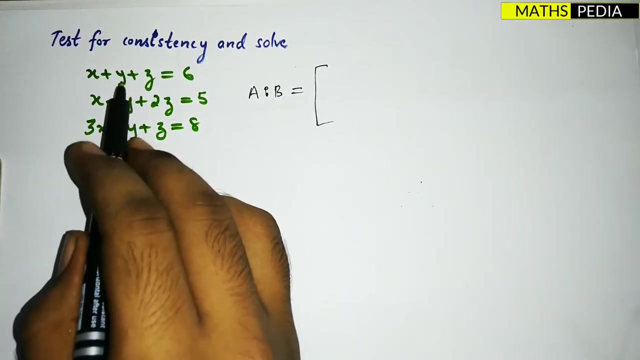 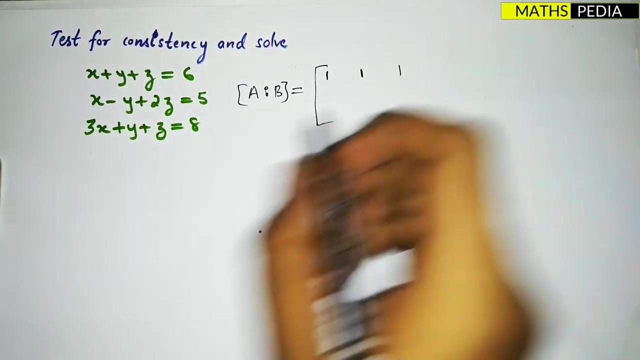 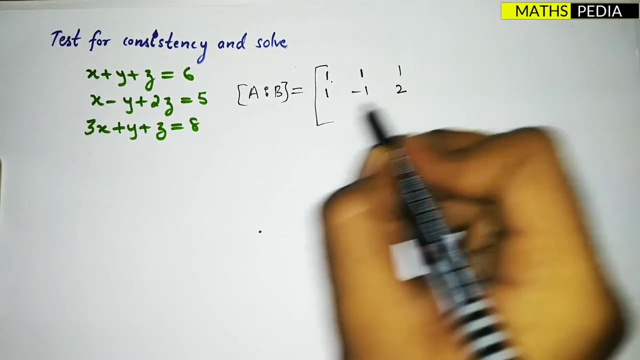 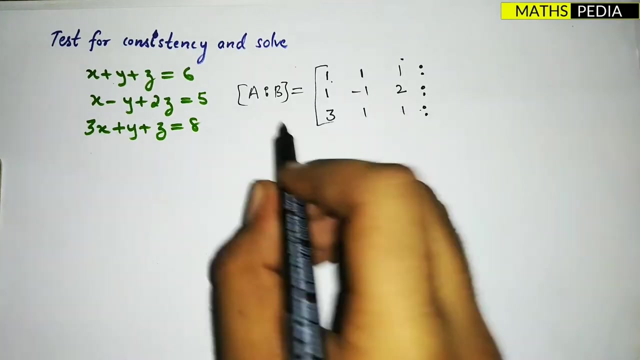 these things. let us start doing the problem. so represent this in augmented matrix. okay, so let us see. that is augmented matrix equal to coefficient of 1, i hope you all know to represent, okay, coefficient of x: 1, 1, 1. okay. next thing: 1 minus 1, 2, 3, 1, 1. and here you have to see the b matrix. b is nothing. 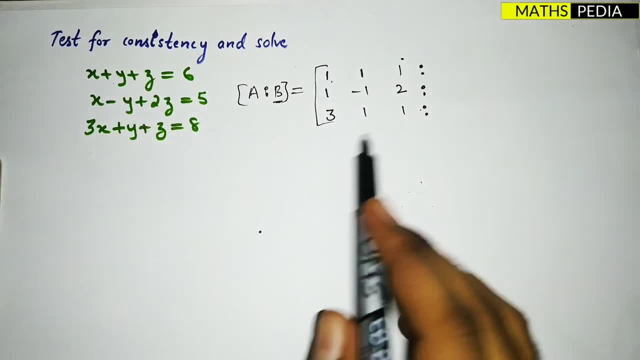 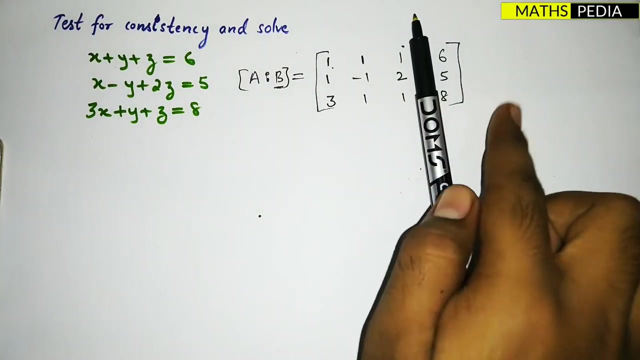 but this one, constants, which should be on the other side r, it's a side, okay, that is 6, 5 and 8.. now, this thing is the first step you need to do. going further for the second step, what you have to do, you have to reduce the a matrix. this is a, okay, this is a and this is b. you have to reduce. 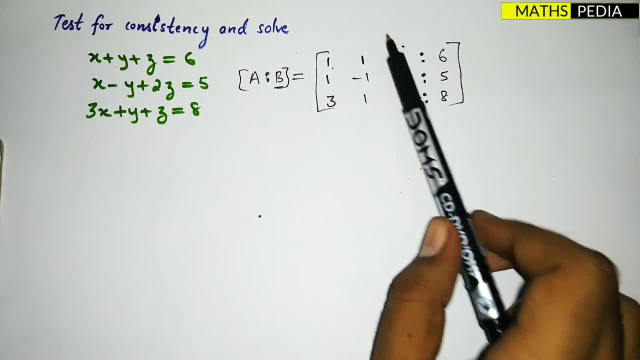 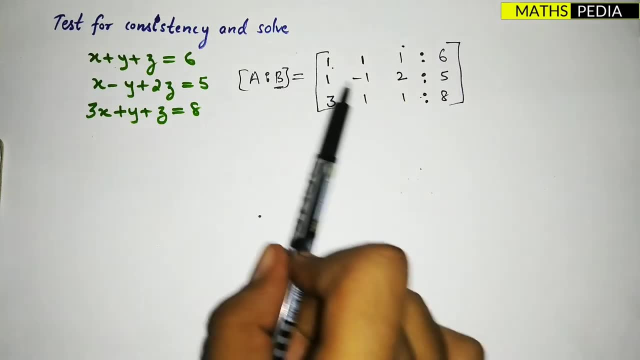 the a matrix into the echelon form. echelon form basically means you have to reduce this as zero, you have to make this as zero, this has zero, this has zero, like that. okay, below the diagonal elements you have to make zero. that means we can see. it is basically upper triangular matrix also. 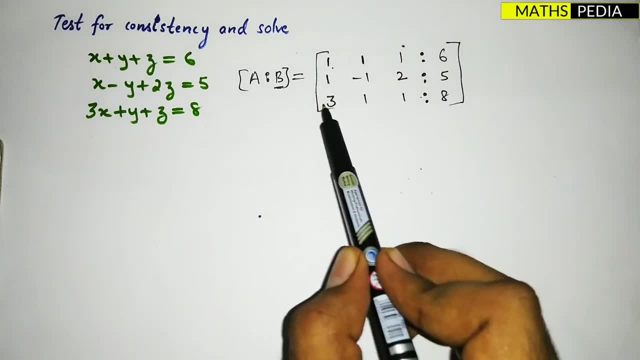 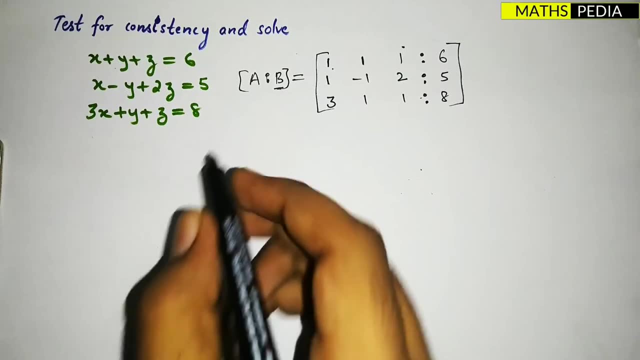 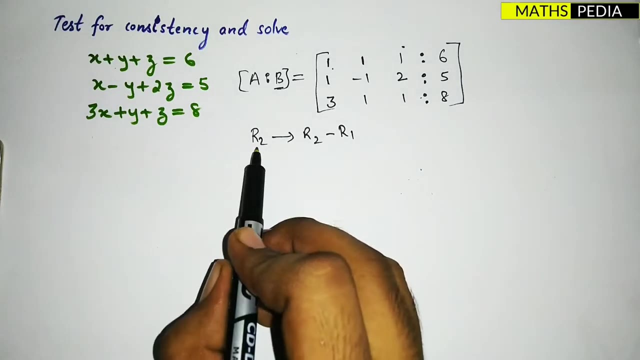 we can see now, you have to do operation on second row and third row in order to make this as zero, and this has also 0.. so what you can do? simply so, r2 is r2 minus row operations. okay, elementary row operations: r2 is r2 minus r1. since it is one, i can reduce it to 0. 1 minus 1 is 0.. so i can do. 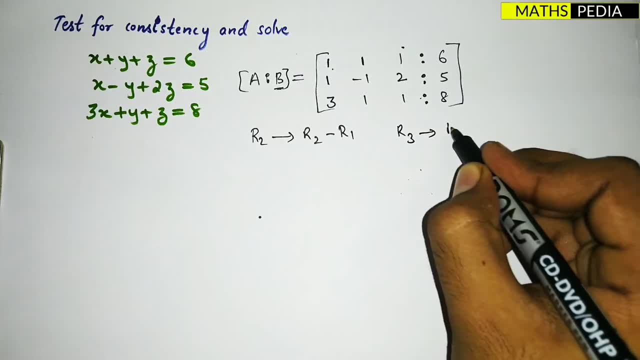 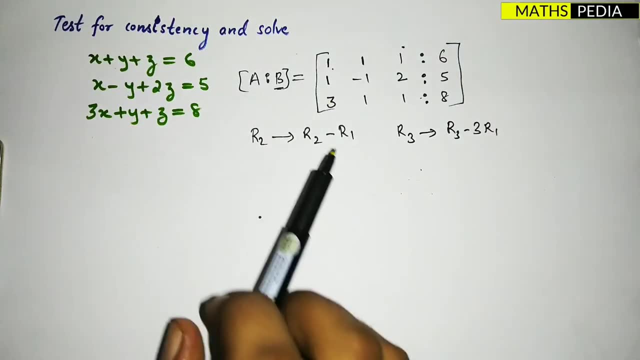 this operation. one more, 4.3.. R3, I can just do R3 minus 3R1.. See 3 into 1 minus this thing. it will be what? 0.. So my intention is to make first this and this 0.. That's it, Okay. So, after doing this operation, 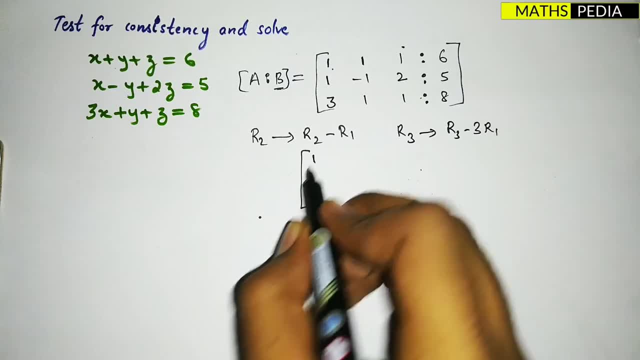 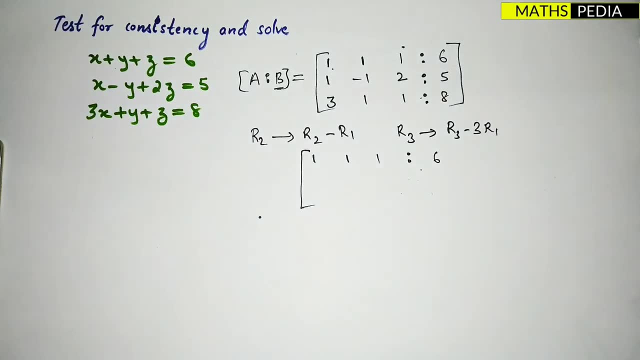 what I will get: 1, 1, 1.. First row will remain as same. Then what happens to the second row? 0, minus 2, 1.. Also remember: here also you have to do operation Okay, But the intention is to. 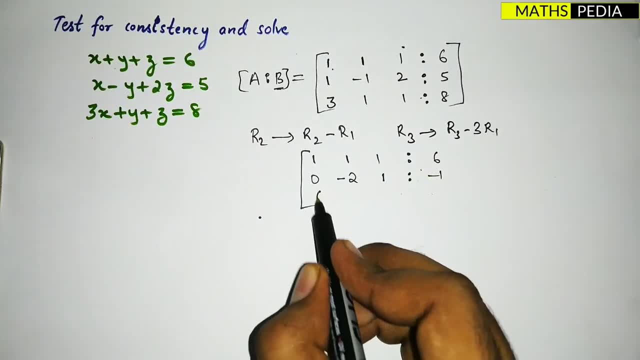 reduce this matrix. Okay, So here, third row, 0, minus 2, minus 2, and here it is minus 10.. Now one more thing: Here also I have to make 0.. Yeah, Correct The diagonal below the diagonal. 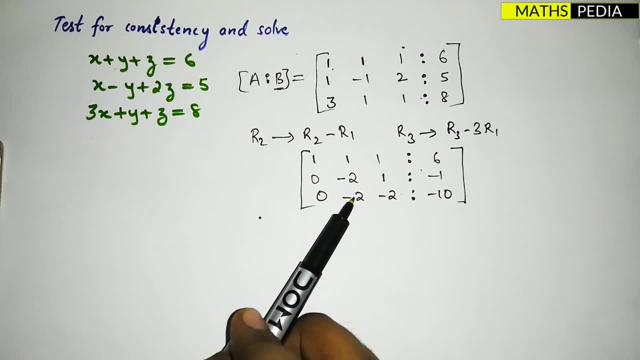 I have to make 0.. So this one I should make 0.. So I can just add, subtract it with this one, Correct, So I can just do one more operation. that is, R3 is R3 minus R2.. Simple In order to make this as 0. 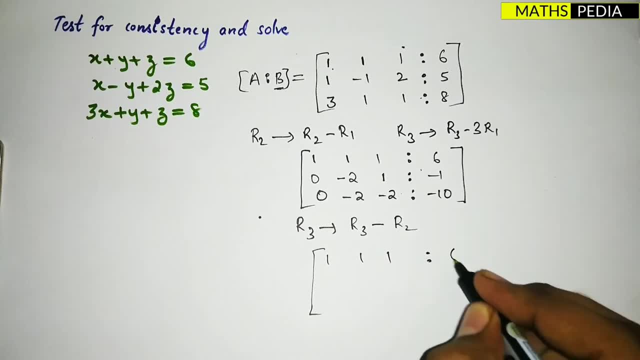 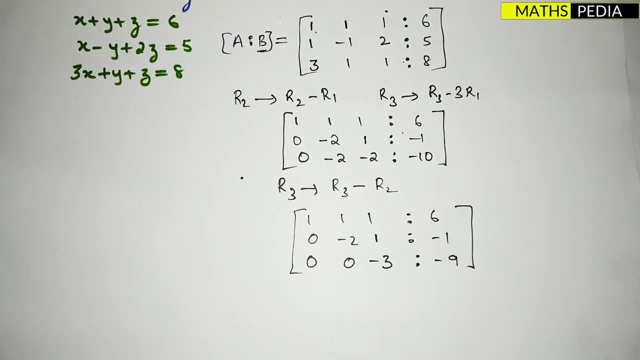 So what will become? 1, 1, 1, 6, 0, minus 2.. Second row: also same, and here it will be: get change. So it becomes like this: Simple. Now the next thing: After reducing it to this one, you need to. 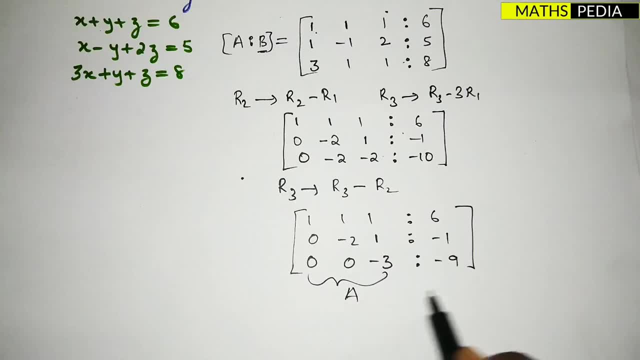 check the rest, So I can just do one more operation. that is, R3 is R3 minus R2.. Simple, Okay. So observe: this is A and this is B. Okay, I hope you know this part Now. here you have to. 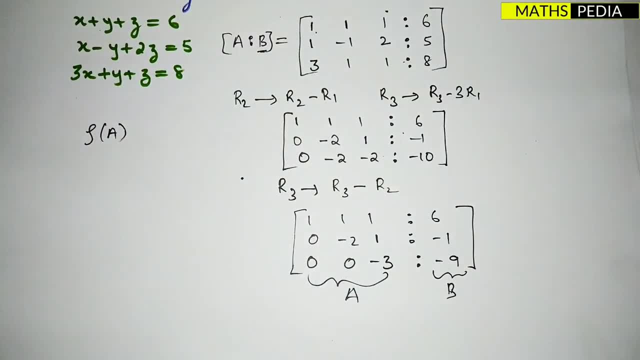 check the rank of A. What is the rank of A? What is rank? Rank of a matrix is nothing but the number of non-zero rows. Non-zero rows, That means here you can see, this is one non-zero row. Here also non-zero row. Here also non-zero. Zero row means what? All the elements should be: 0.. Okay, 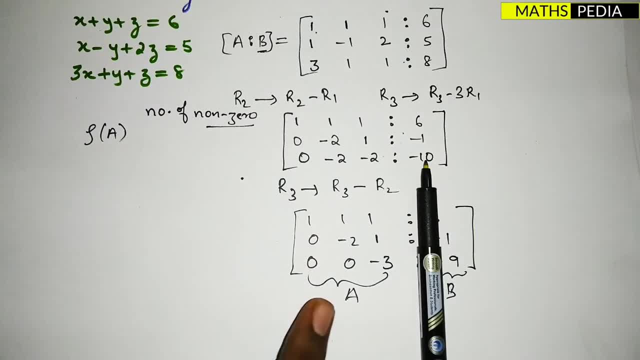 So only see the A matrix. Here you have to check the rank. You can observe that there are three number of non-zero rows. Don't see this one, Don't think that here zeros are there. Then it is 0.. Okay, This is. non-zero rows means this one, Any of the element. if it is non-zero, then that row is. 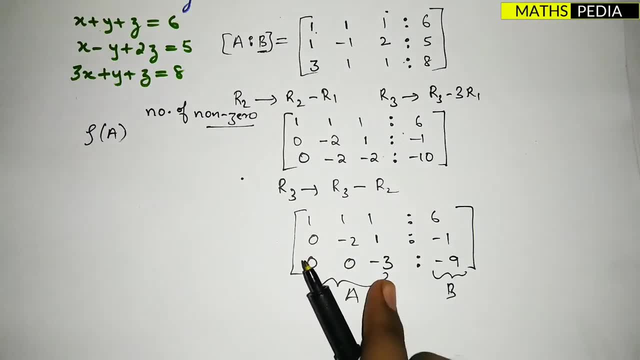 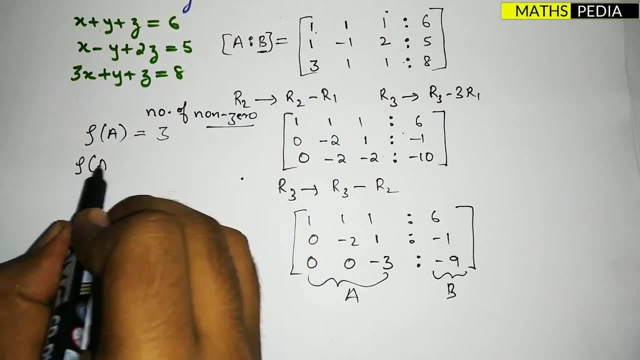 non-zero row. That's it Here. it is minus 3.. So it is non-zero row 3.. So rank will be 3.. I am talking about matrix A only. Okay, Now we will talk about augmented matrix AB. Rank of that means the whole thing, Whole thing. 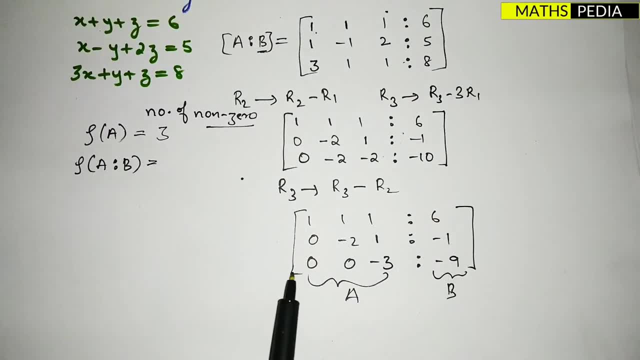 you have to see. Here you can see this is non-zero row, Non-zero row, And here also we can see it is non-zero row. Okay, The whole thing you have to see Here also, it is 3.. Number of non-zero rows. 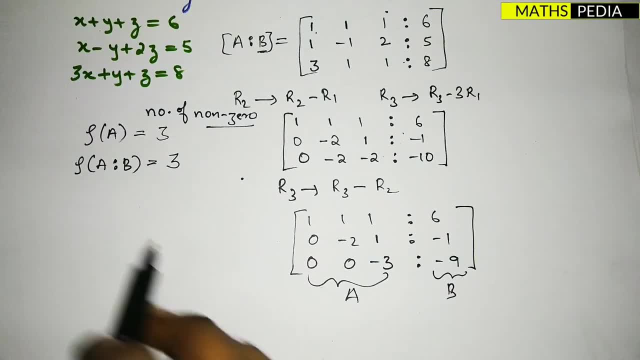 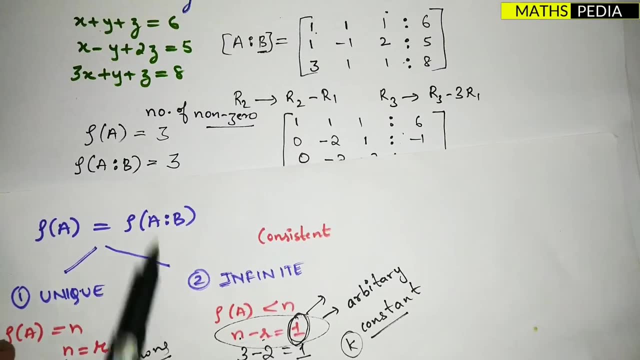 That means it is a rank of that particular matrix. Now we got these two things. Now you have to just check. You can see earlier I have discussed this part. See, both are equal. Then what is the case? When both are equal, then it is consistent. So we got that, whether it is. 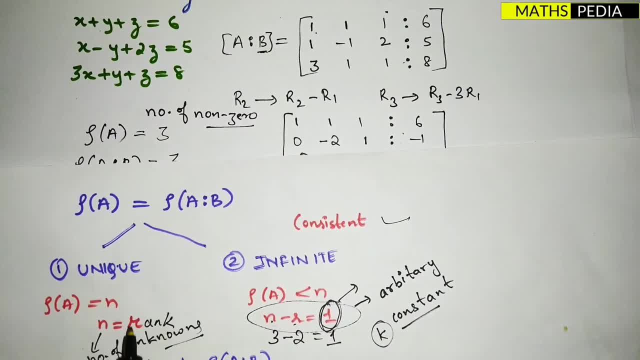 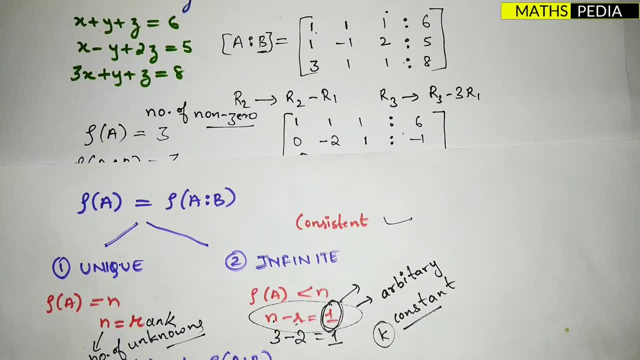 consistent or inconsistent. So hence it is consistent. Now we have to check for the unique solution, whether it has unique solution or infinitely many solutions. So for that, what you need to do, You have to see whether it is equal to number of unknowns, Rank of A or rank. 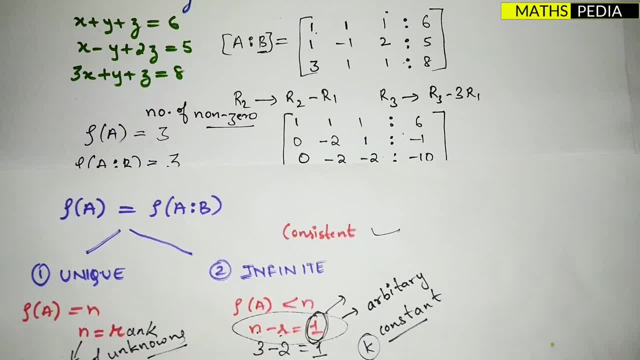 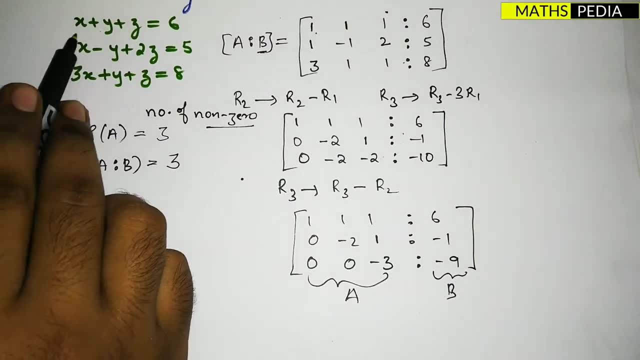 of both. Anyways, both are equal. Whether it is equal to number of unknowns or whether it is less than that We will see. Number of unknowns basically means what You can see for the question X, Y, Z: How many unknowns? 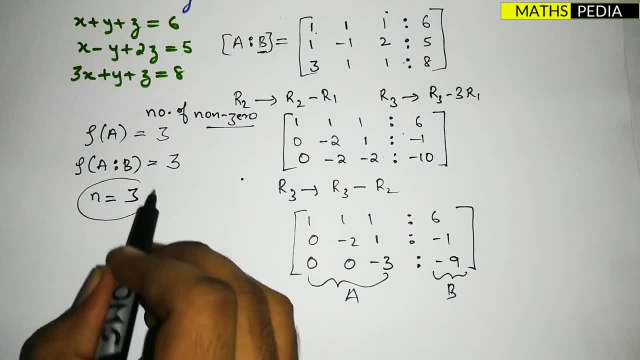 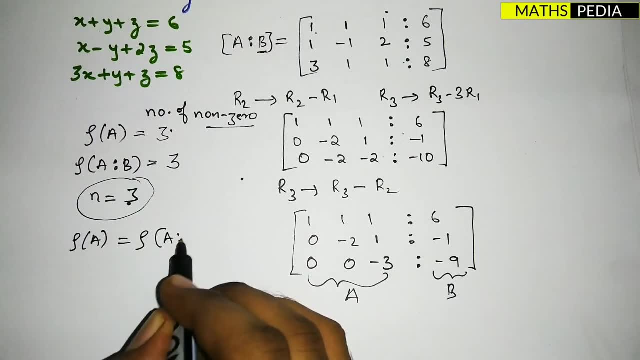 are there 3.. That's it. So N is equal to rank, correct. See here, Rank of A, which is equal to rank of this one, which is equal to N, correct? So therefore, we can say what It is consistent. 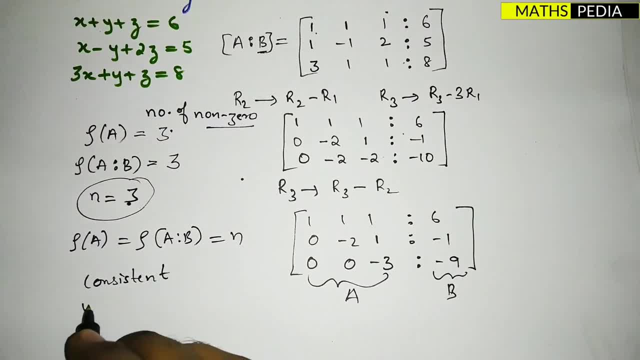 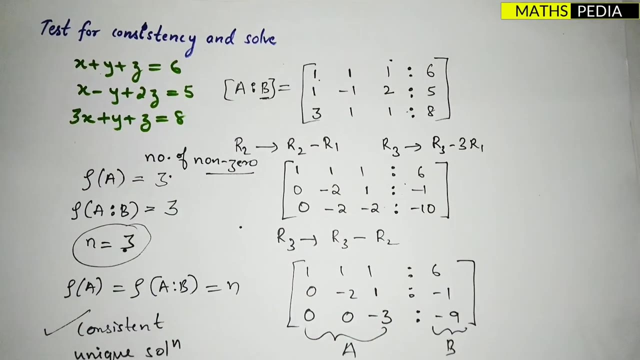 and unique solution. Okay, So hence we have proved that it has unique solution and it is consistent. Now we need to find the solution of that. How to find? Because it is asked to find solve also. That means you have to find the solution of that. 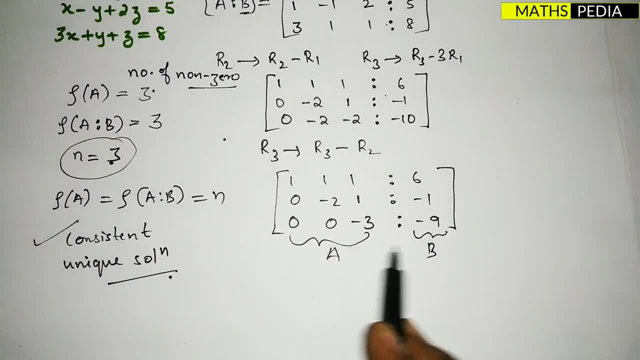 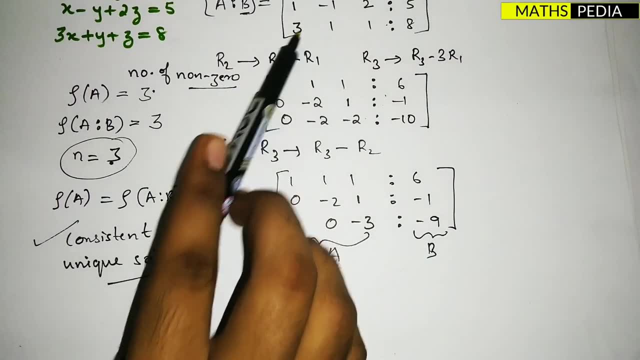 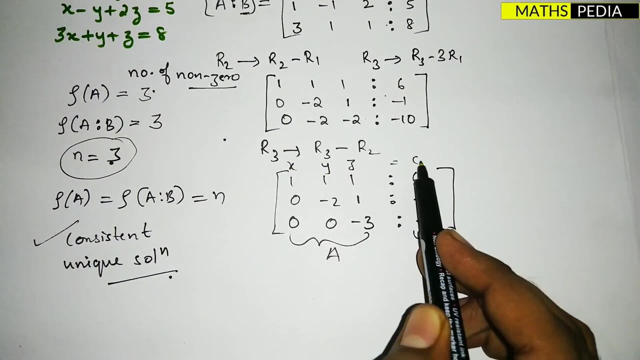 How to do that. Let us see So from here, from this matrix, that is augmented matrix, the last step you have to form the equation from this, Not from the first step. okay, X plus Y. I hope you know. this is X, this is Y and this is Z and this is. we can see the constant part, So we can. 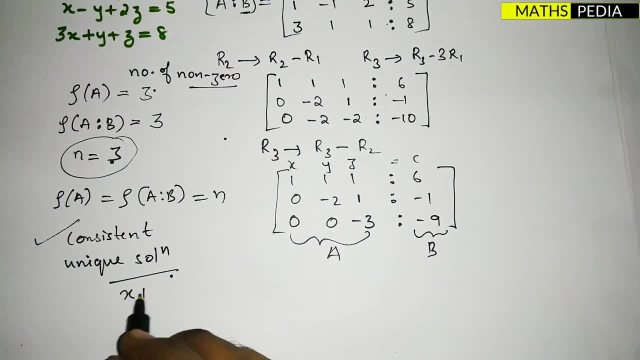 find the equation from this, So I can say it is equal to what? X plus Y plus Z, which is equal to 6, this equation, Next one, 0X. no need to write Minus 2Y plus Z, which is equal to what is the? 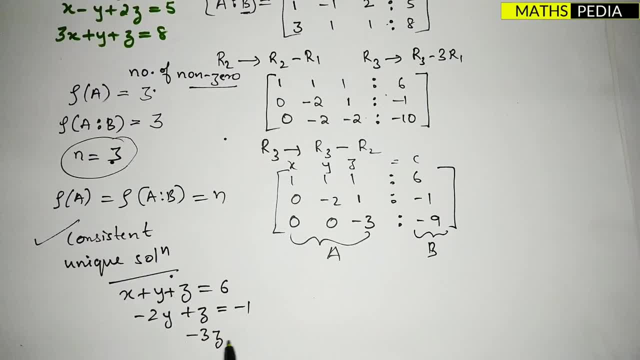 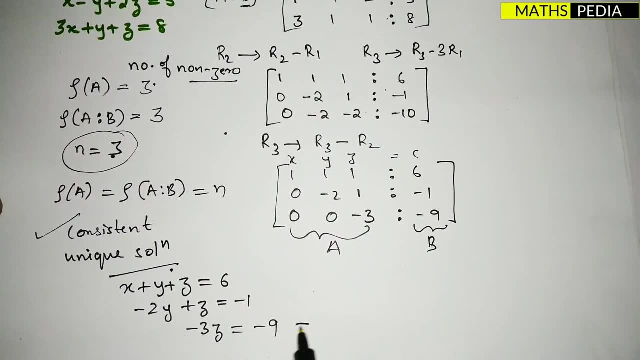 constant here Minus 1. and one more thing: minus 3Z is equal to minus 9.. So minus 3Z is equal to minus 9.. So we can directly say from this: Z is equal to what. 3, correct, Now Z is equal to what.